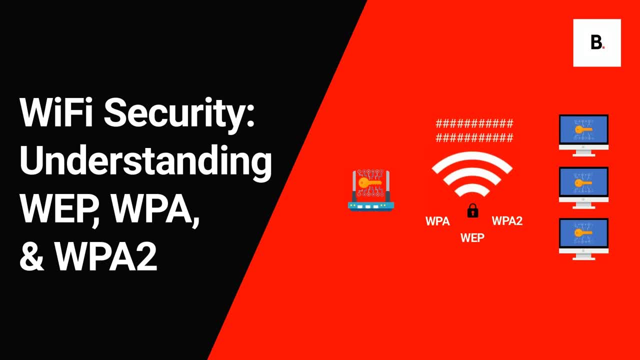 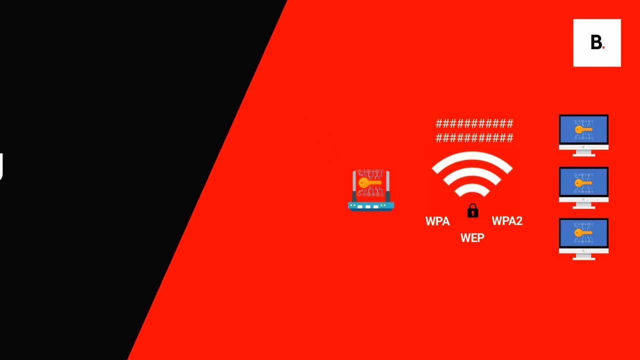 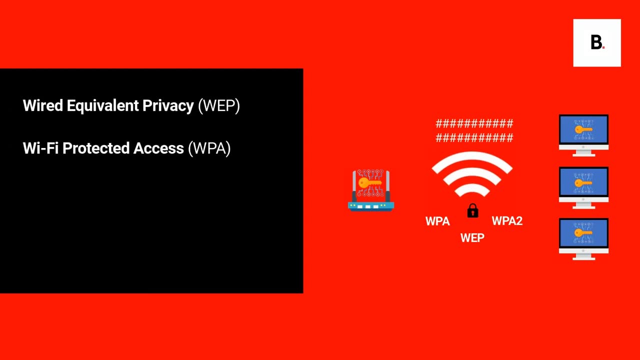 meaning the same key is used to encrypt and decrypt data. The Wi-Fi Alliance, a non-profit organization which owns the Wi-Fi trademark, certifies all Wi-Fi security protocols. There are four Wi-Fi security protocols currently available: Wired Equivalent Privacy, Wi-Fi Protected Access, Wi-Fi Protected Access 2, and Wi-Fi. 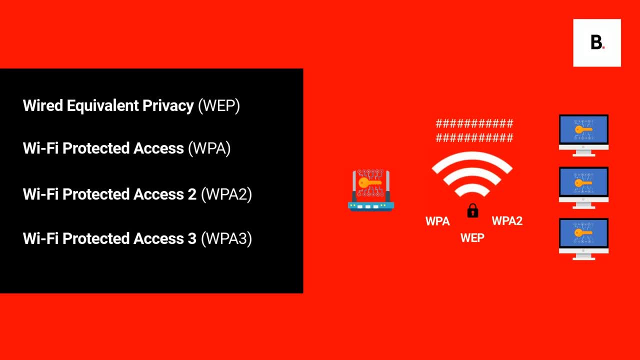 Protected Access. 3. Wi-Fi networks transmit data through radio waves, meaning data can be easily intercepted unless security measures are in place. If your Wi-Fi is left unsecured, hackers could steal your internet bandwidth, monitor your internet activity, carry out illegal activities through your connection and install malware on your network. Therefore, 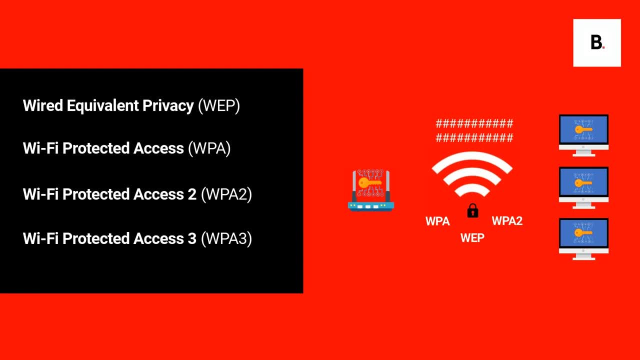 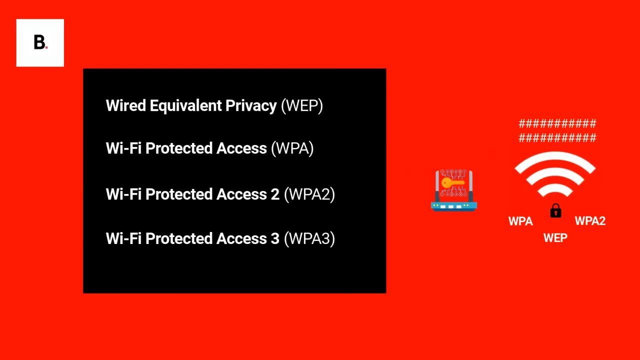 it is vital to understand the differences between these security protocols and implementing the most advanced one your router can support. Let's take a look at each of these wireless security protocols in more detail. Wired Equivalent Privacy was introduced in 1997 and was the first attempt at wireless. 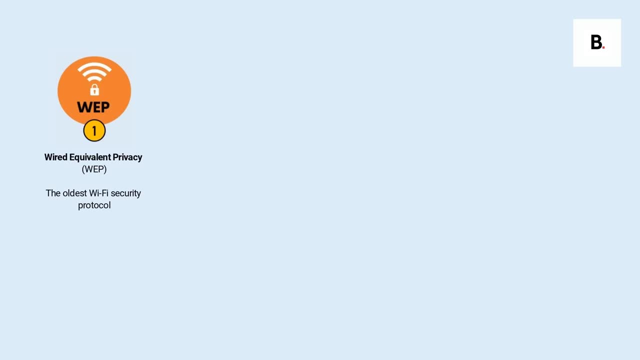 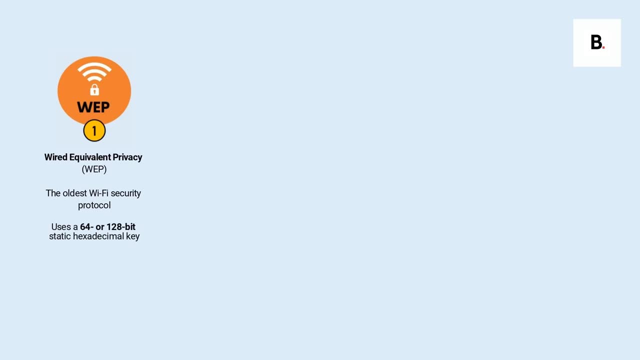 static exodecimal key. This means all traffic is encrypted using a single key, regardless of the device. Despite revisions to the protocol over time, several security vulnerabilities were found in the WEP standard. The increase in computing power also made it easier for 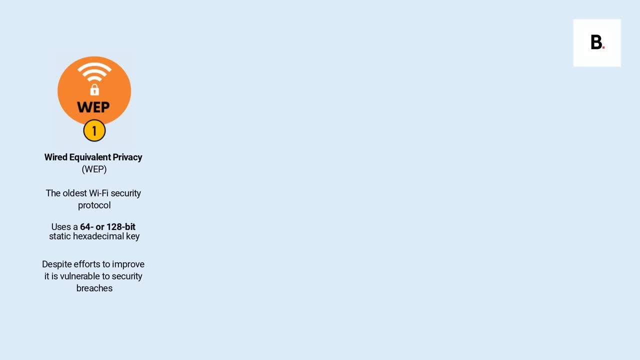 cybercriminals to exploit these flaws. Because of this, the Wi-Fi alliance officially retired WEP in 2004.. Today, WEP security is considered outdated and rarely used. Introduced in 2003,, three WPA or Wi-Fi protected access quickly replaced of WMP. While WPA shares similarities, 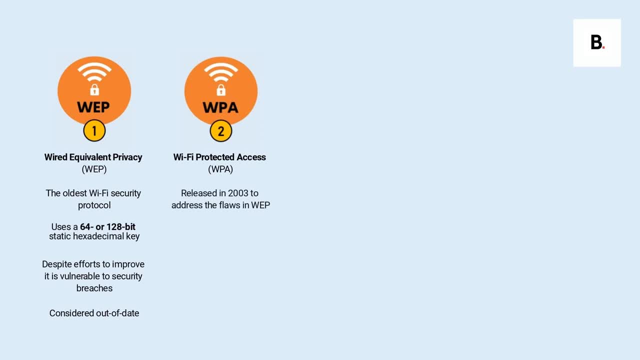 with WEP. it offers improvements in how it handles security keys and manner in which users are authorized, Whereas WMP provides the same key. each authorized system. WPAs uses TKIP or Temporal Key Integrity Protocol, which dynamically changes the key used by the systems. WPAs also checks 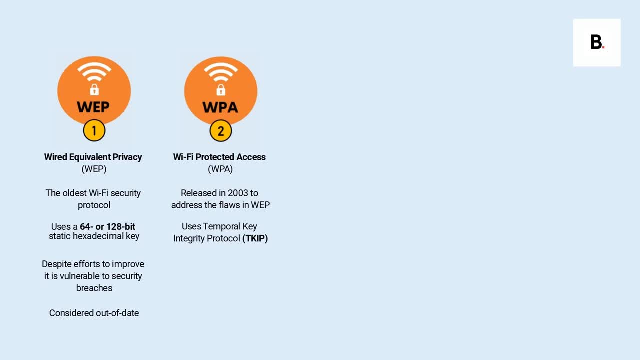 message integrity. to identify if data packets have been captured or altered by a hacker, WPAs uses 256-bit keys as opposed to the 64-bit and 128-bit keys used in the WEP system. However, despite these improvements, components of the WPA Wi-Fi security protocol can be exploited. 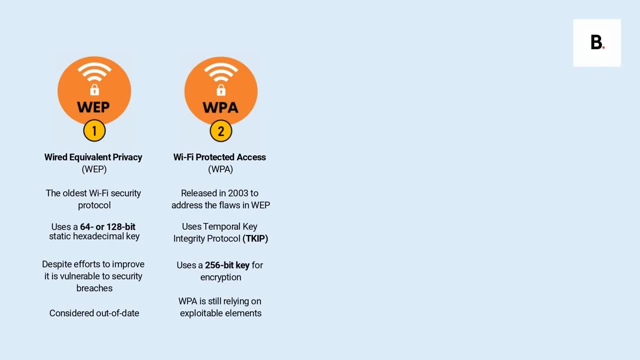 needing the standard to be further revised. Wi-Fi Protected Access 2, or WPA2, is the second generation of the WPA Wi-Fi security protocol aiming to secure Wi-Fi network. Data transmitted and received over your wireless network using the WPA2 standard is encrypted. 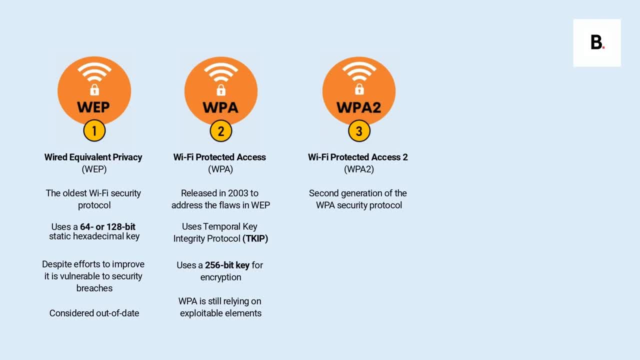 and only people with your network password have access to it. WPA2 uses the Advanced Encryption System, ADS. compared to the less secure TKIP system used in the original WPA protocol, ADS provides strong encryption and is used by the US government to protect classified data. 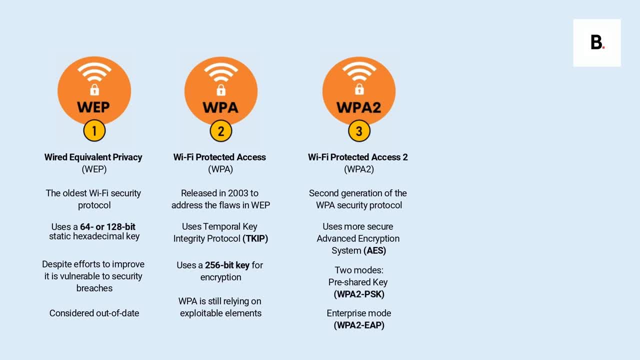 WPA2 operates in two modes: WPA2-PSK or Personal Mode, or Pre-Shared Key, which uses a shared passcode for access and is usually used in home and small office environments. WPA2-EAP or Enterprise Mode is more suited to organizational or business use. 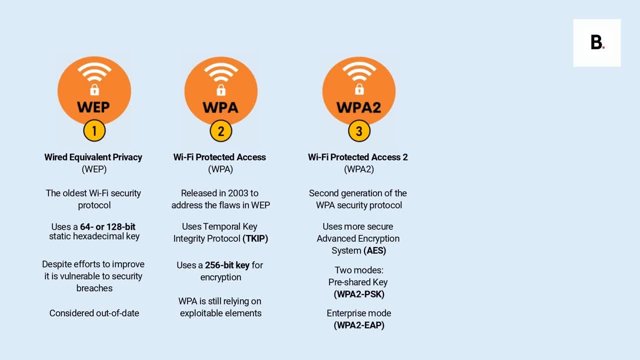 requiring a RADIUS server to authenticate users. Like its predecessor, WPA2 components such as routers are vulnerable to attacks through WEP. Consequently, when deploying WPA2, it is advisable to disable WEP and, where possible, make sure your router's firmware doesn't rely on WEP. 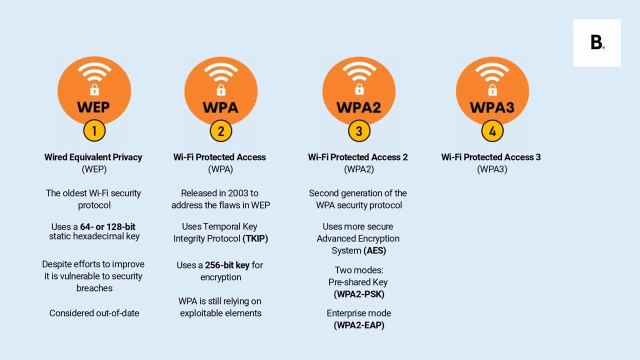 Introduced in 2018, WPA3 introduced new features for both personal and enterprise use, such as individualized data encryption, simultaneous authentication of equals protocol and stronger brute force attack protection. WPA3 uses perfect forward secrecy to encrypt data, making it more secure than its predecessor, WPA2.. However, WPA3 has not been widely adopted yet. 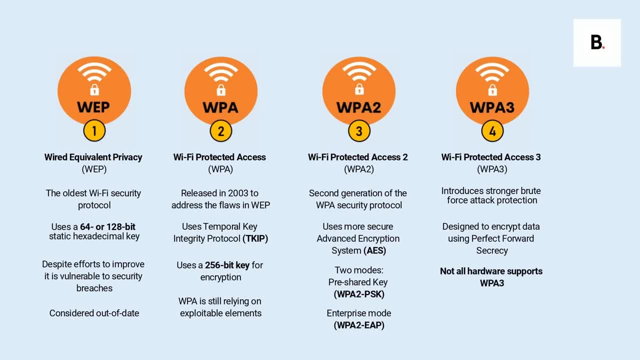 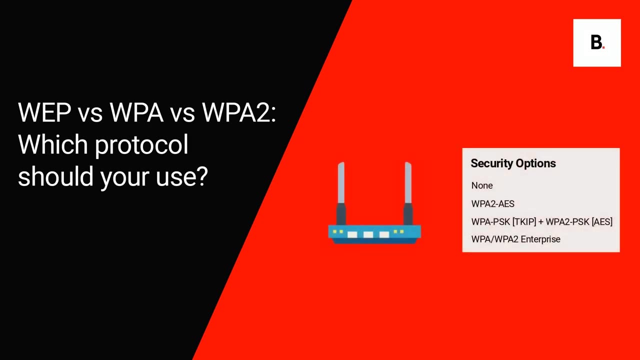 and not all hardware supports WPA3 automatically, While using this protocol may require costly upgrades. WPA3 devices are backwards compatible with devices that use the WPA2 protocol. Which Wi-Fi security protocol should you choose? The WEP Wi-Fi encryption standard is now considered outdated. Most modern routers will not even.